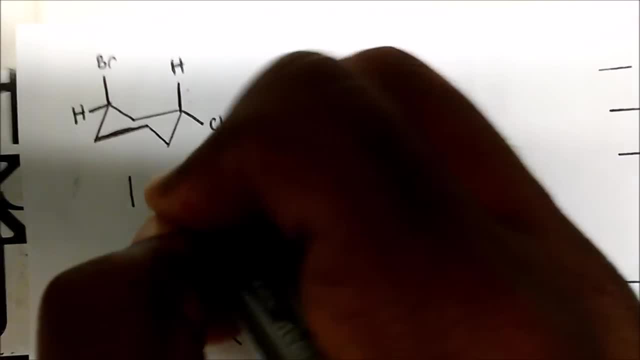 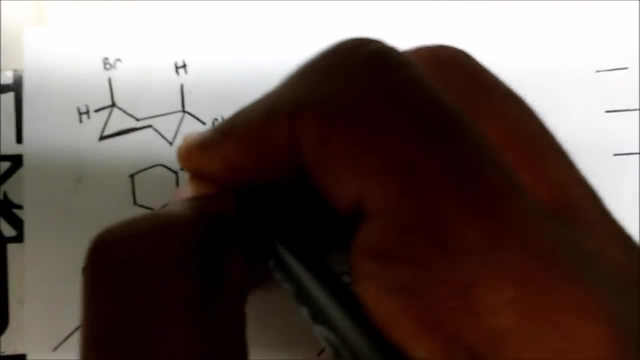 All right. so really we have a cyclohexane And on carbon 1, the chlorine is going down, which kind of usually means that we have a dash. So on carbon 1,, 2,, 3,, 4, 5, the bromine is actually. 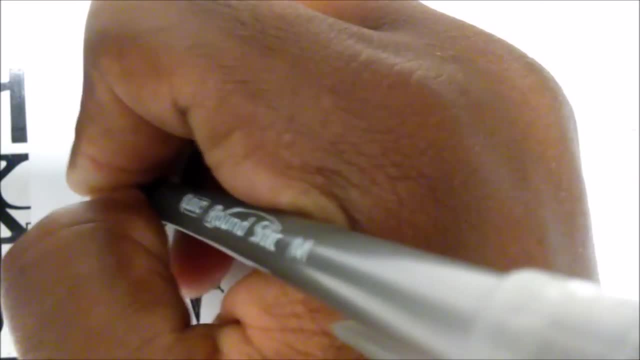 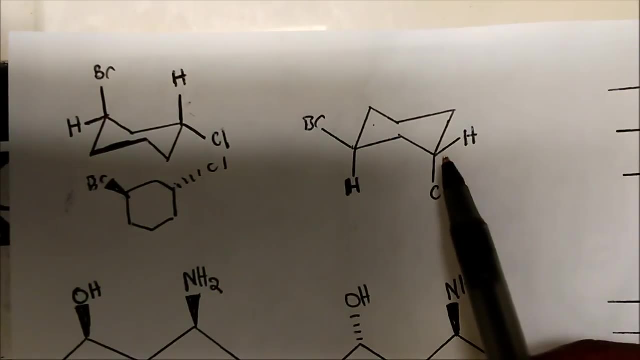 going up, which means that the bromine kind of have this kind of cis thing to it right Now. how about this? This looks like a different chair conformation, but let's see. On carbon 1: now we have the chlorine going down, So this will now be carbon 1.. So 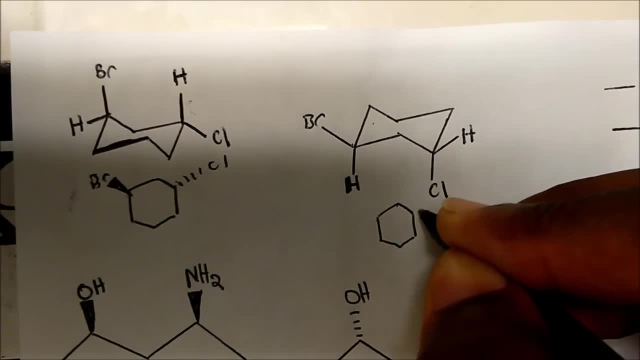 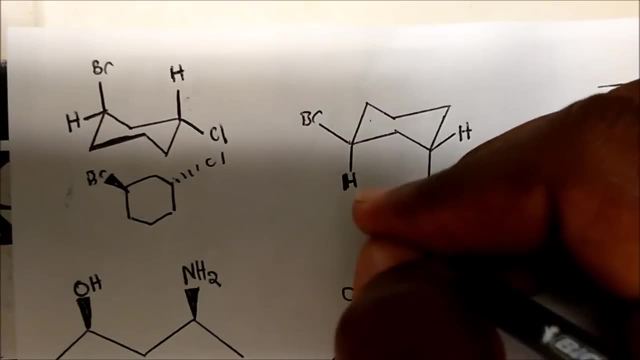 again on carbon 1, we have the chlorine still going down. Carbon 1,, 2,, 3,, 4, 5, we have the bromine. It's going up On carbon 5, the bromine is going up All right and, as you could see, 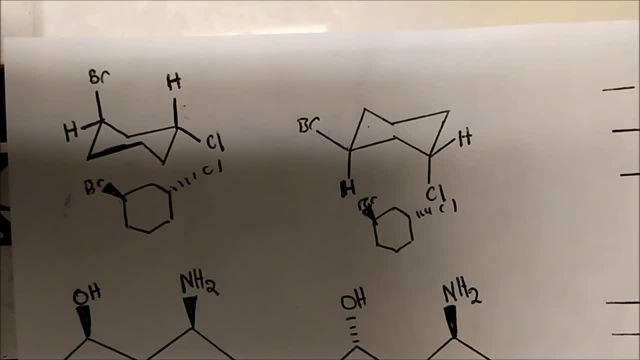 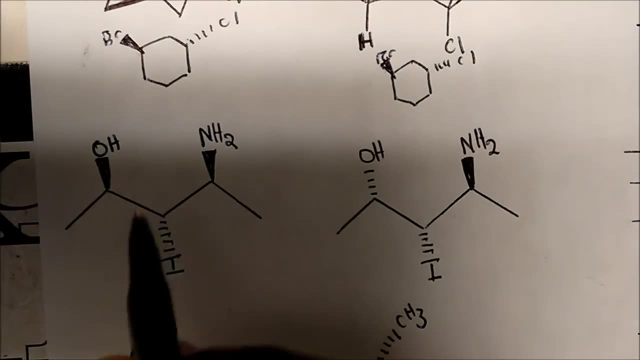 these are the same molecules, literally the same thing. These are just the chair conformations flipped, So these are identical. Let's look at the second pair of molecule here. All right, so how many chiral centers we see? We see three different chiral centers. Now look closely. The OH group changes right The ID. 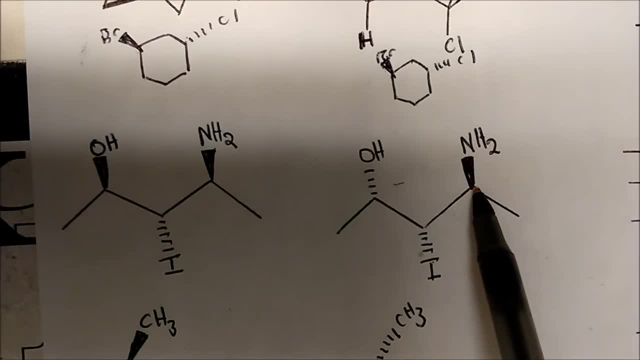 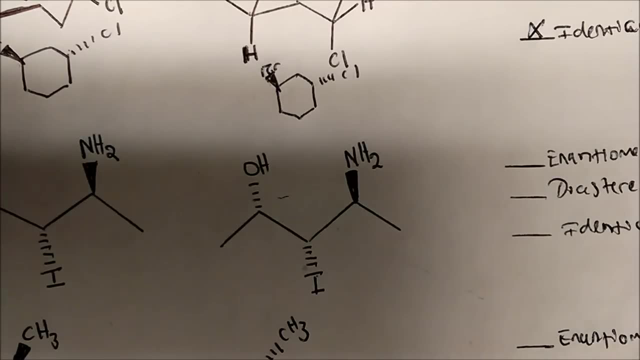 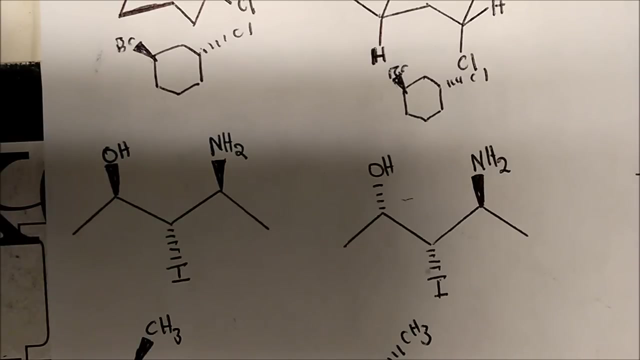 group stays the same. The NH group stays the same, right, So there's only one thing that changes in the molecule, And in this case we'll classify these diastereomers. And the reason that a diastereomer, how it differs from enantiomers, is that it has to have at least two. 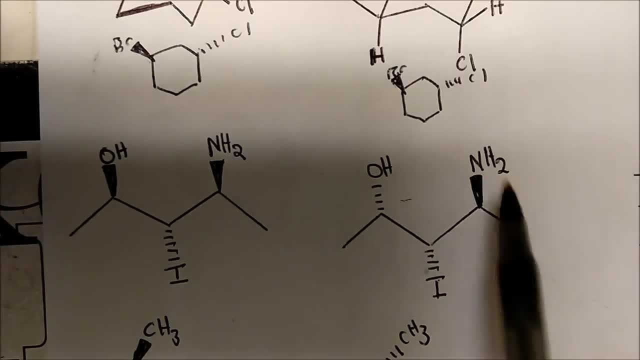 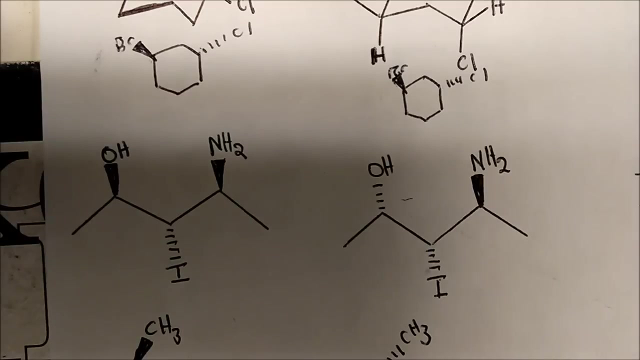 chiral centers, with one staying the same. So notice that our amine group stays the same, right, They both have wedges. and our iodine group stays the same- They both have dashes. However, our OH group changes. Well, we have two chiral centers. that pretty much stays the same. 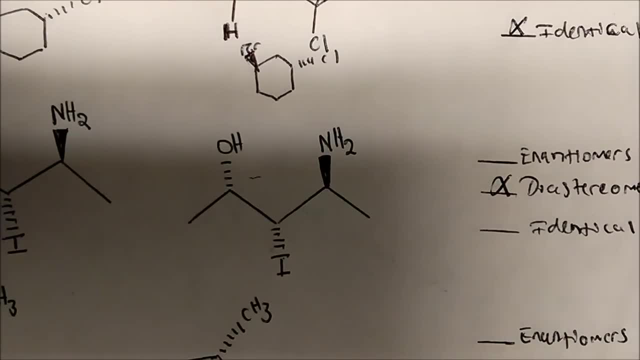 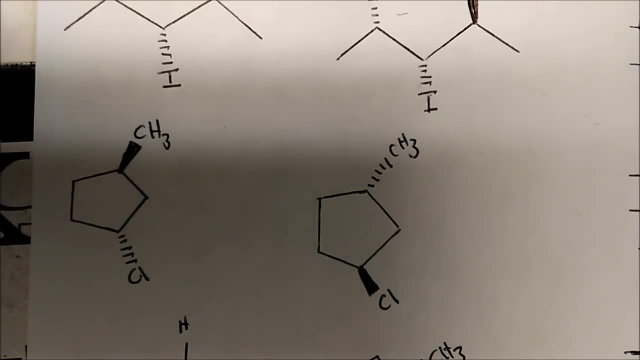 but one changed, And so that is what we'll classify as a diastereomer. How about this one? What would be the classification of this molecule? Well, again, we notice that there are two chiral centers in the molecule. But notice how your chiral centers changes, right. So over here. 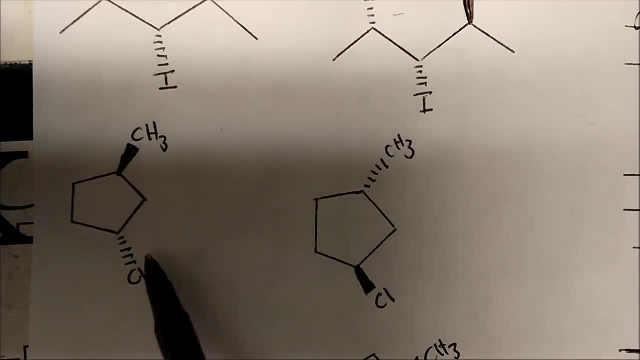 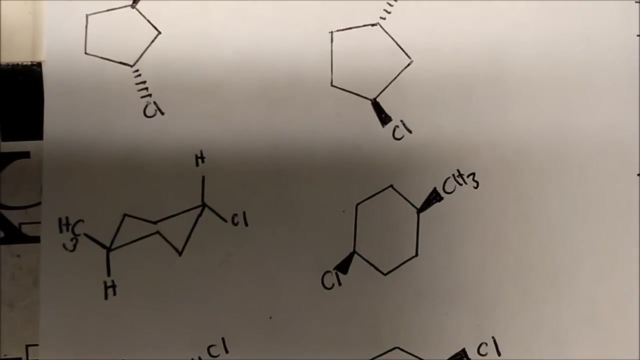 we have a CH3 that went from a wedge to a dash. We have a chlorine that went from a dash to a wedge. Anytime you have all your chiral centers changing in such fashion, that will always give you an enantiomer. All right, let's look at this one. 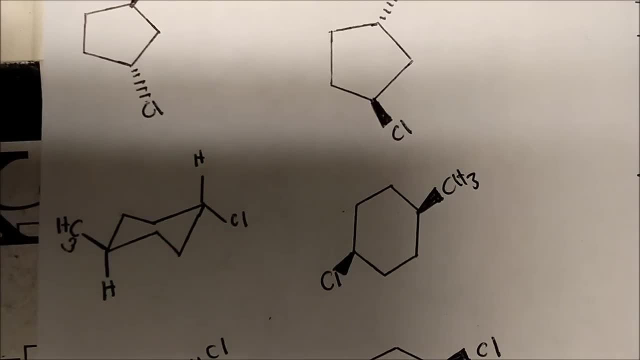 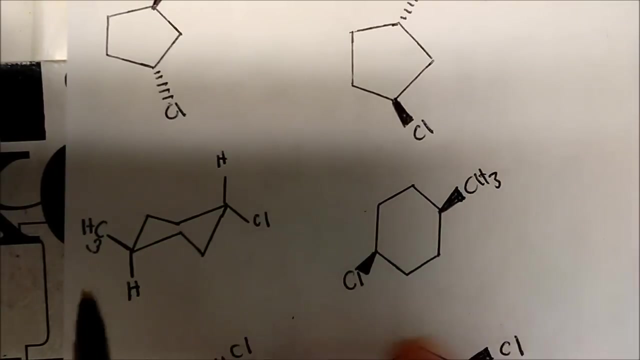 We have this cyclomethylchlorocyclohexane right here, right, And then we have this chair conformation of the molecule. Well, let's see, We could call this carbon 1.. And as you can see, in carbon 1, here we have the CH3 that is basically going up or kind of coming. 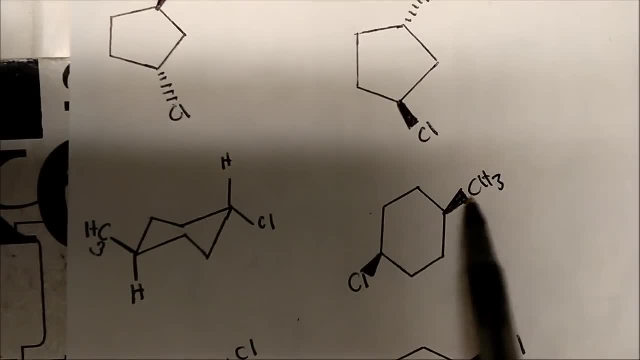 out at us And this is consistent with what is here. right, We have a CH3 that's coming up or kind of coming out of us. right On carbon 1,, 2,, 3, 4, right So on carbon 4,. so 1,, 2,, 3, 4, we have the chlorine group. that is. 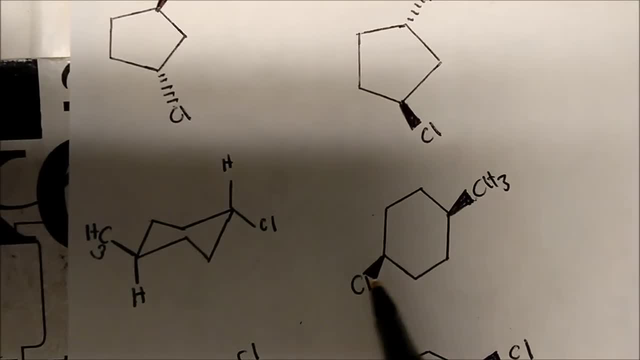 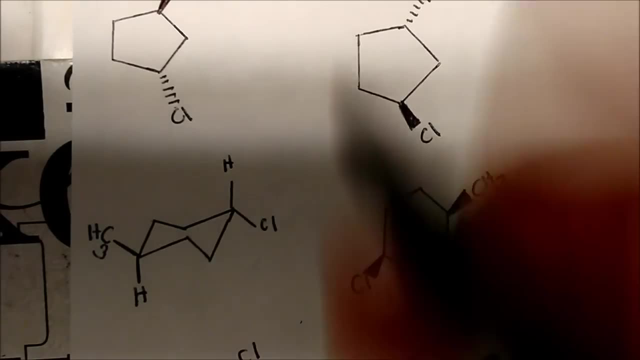 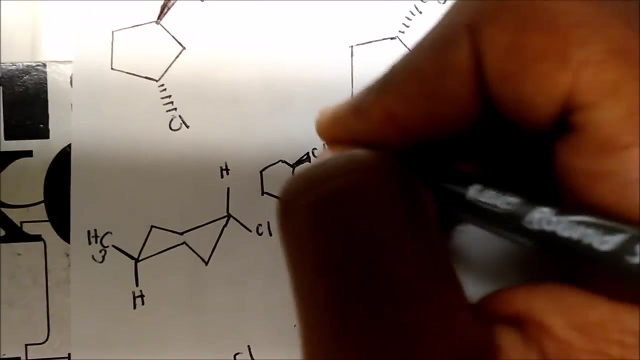 actually going down. right, Here the chlorine group is coming out at us, right, So the chlorine group is coming out at us, Here it's going down. So this is basically this now have. so the molecule looks something like this: right, The CH3 group stays the same because it's coming. 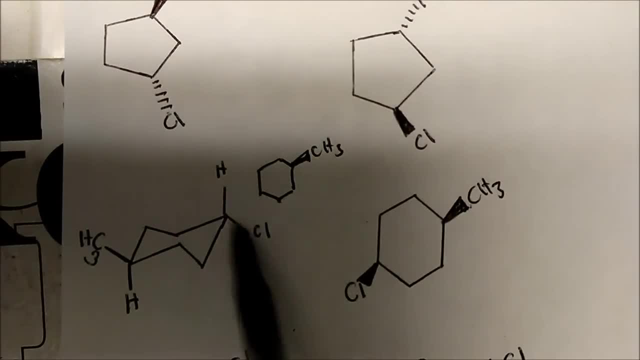 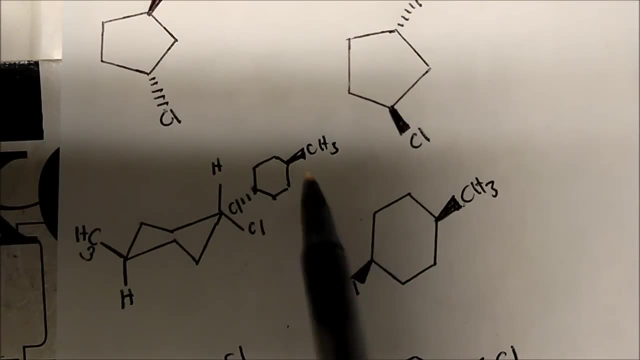 out of us right. So on carbon 4,. now the chlorine is going away, which means that it has a kind of dash right. So looking at these two molecules here, we can see that one, chyrosanit, stays the same. 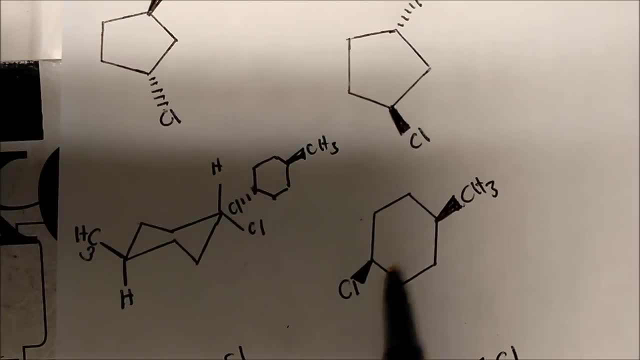 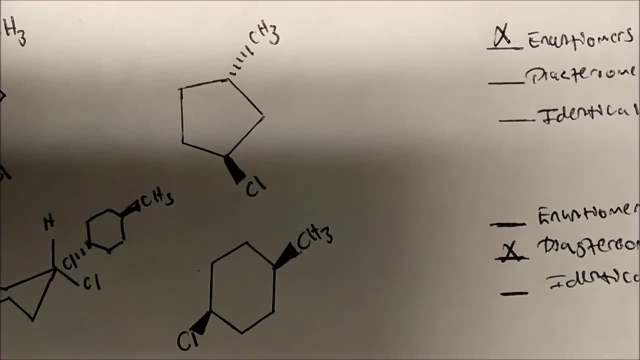 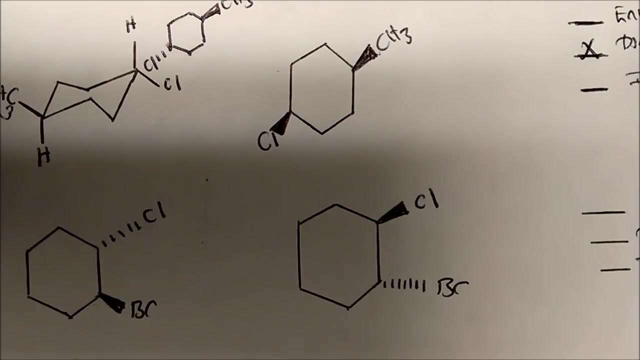 but the other chyrosanit, switches right. This now one chyrosanit stays the same, but the chlorine switches right, And this, again, is what we classify as diastereomers. How about this one? Well, looking at this molecule, notice that both are chyrosanit changes. 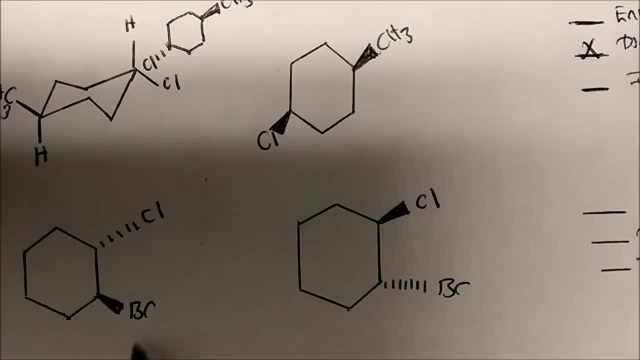 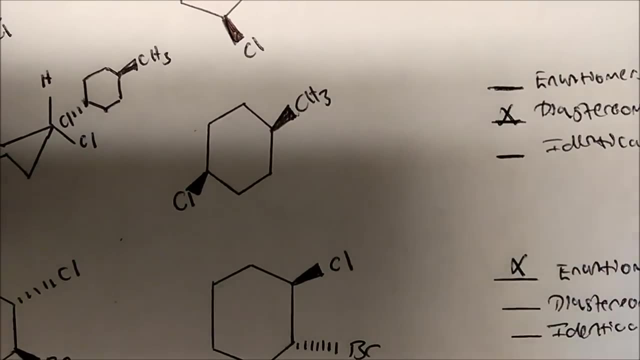 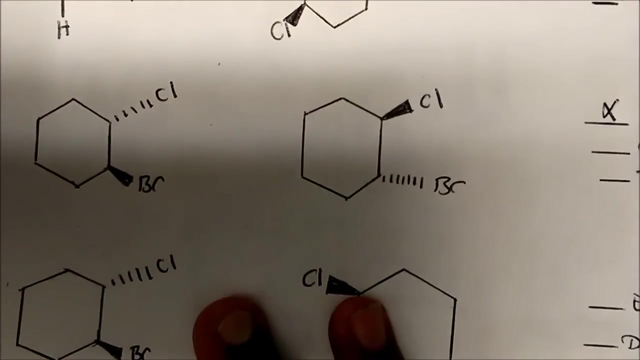 So the chlorine goes from a dash to a wedge and the bromine goes from a wedge to a dash right, And this is simply a nanotumor. All your chyrosanit is changing. That's what we classify as a nanotumor. All right, how about this one? All right, how about this one? How about this one? 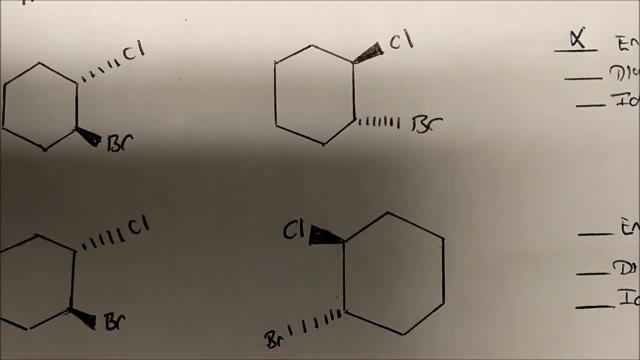 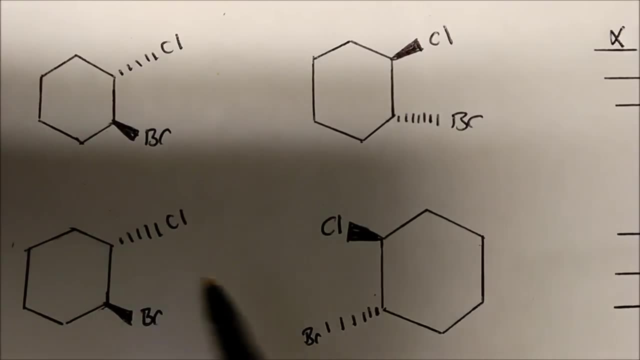 All right, we have this molecule, this paramolecule, here, all right. So again here we have a chlorine going away and the bromine having a wedge. But here, look, the molecule is flipped and now the chlorine is going away. 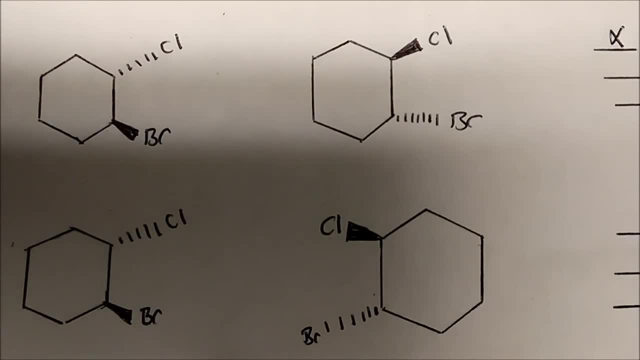 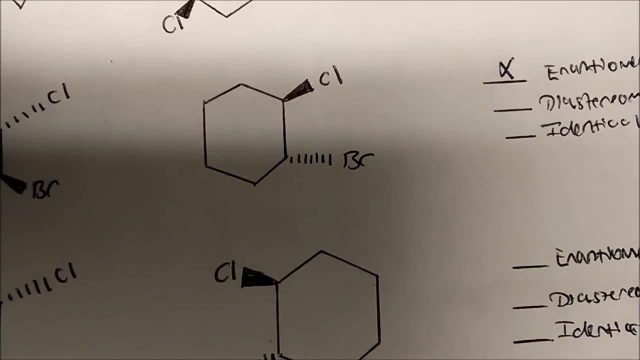 The chlorine is coming out at you, the bromine is going away. The reason why I put these two together? because I want to illustrate something here: These and take your basket and you could pause this video, but these are actually identical. 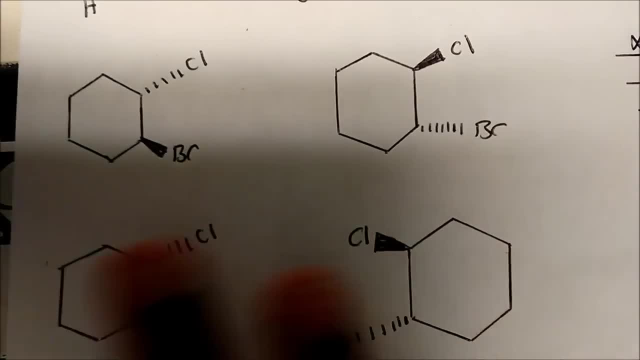 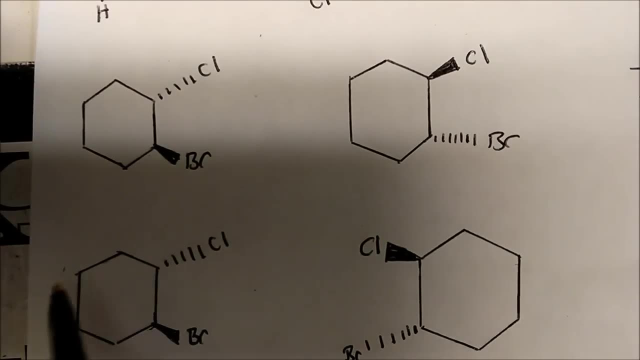 These are the same molecule and what you find out is that if you were about to take this molecule and flip it over, you would see that your chlorine- that was going away from you- will be coming out at you, and your bromine that was going away from you- that was coming out at you- will be going away from you, which is exactly what. 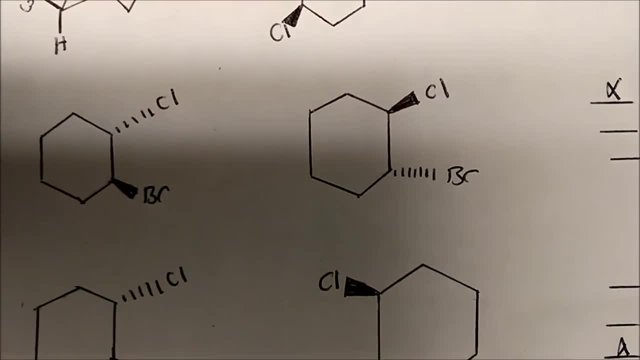 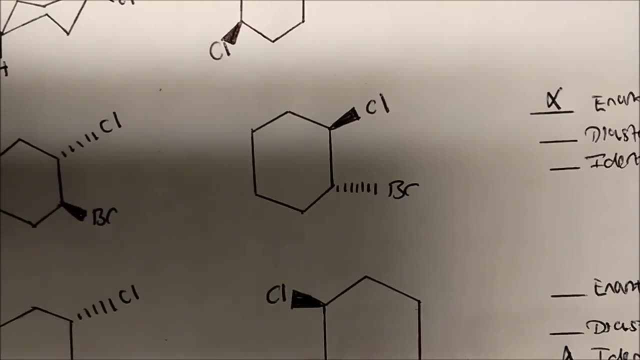 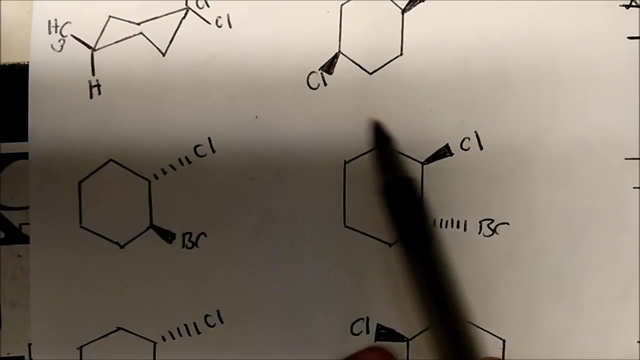 you see right here, and it's just the same molecule flip. now you could draw enantiomers two different ways. right, you could draw enantiomers two different ways, and this is one. this is what i wanted to illustrate this. these two enantiomers notice that the substituents are on the same side, but 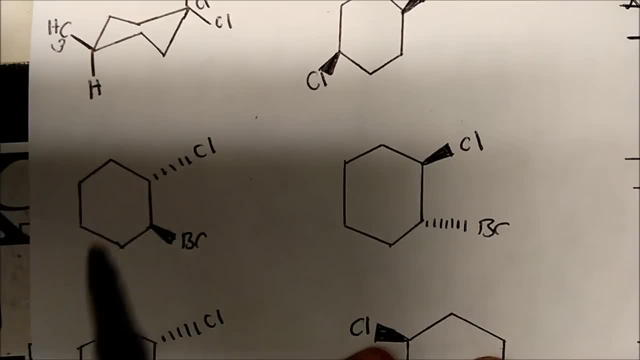 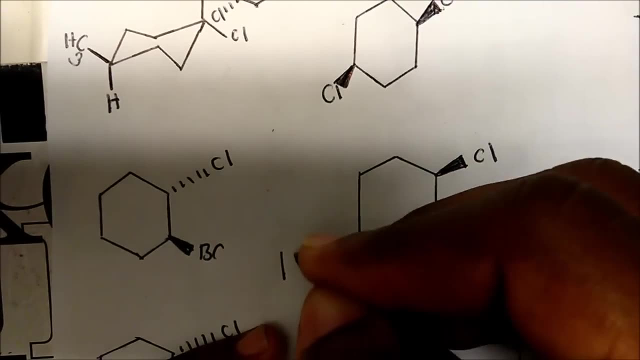 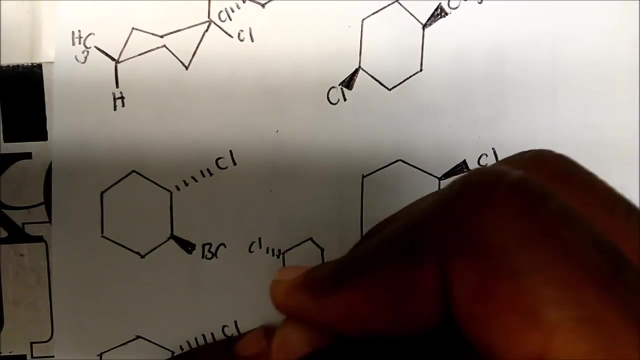 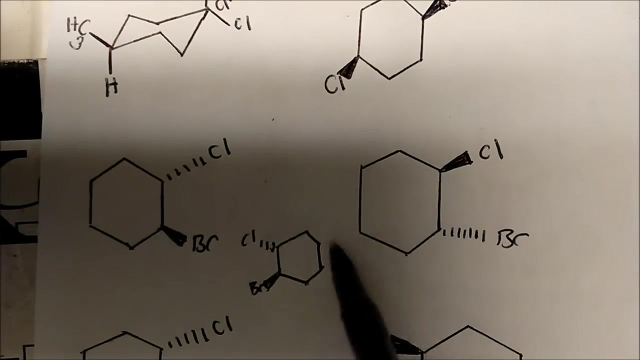 the carlsen, it changes. that's one way of drawing an enantiomer. another way of drawing an enantiomer of this compound- and i'm going to squeeze it in here- is something that looks like this: so this, these are two enantiomers of this compound here. notice the difference between this and this. 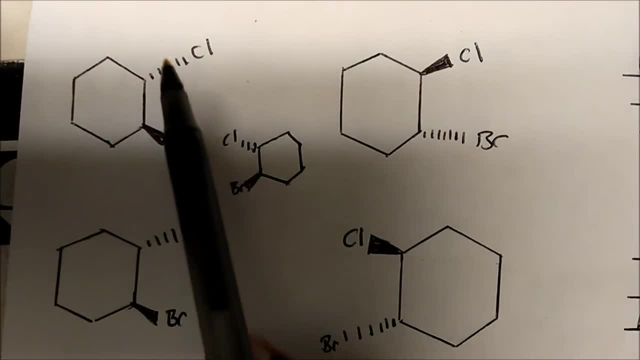 right here. the molecule flips, but the carl center never changes. the carl centers are the same, and once you find out that these two are non-superimposable on each other, right, they're non-superimposable on each other. on this end, when you flip the molecule, 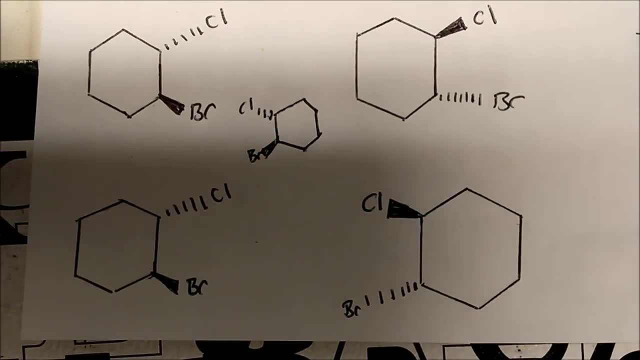 the carl centers change, right, and that is just just saying that you all your doing is just flipping the molecule and and that will give you the same identical molecule- flipping the molecule, but you got to keep your carl centers to change. that's the same if you. 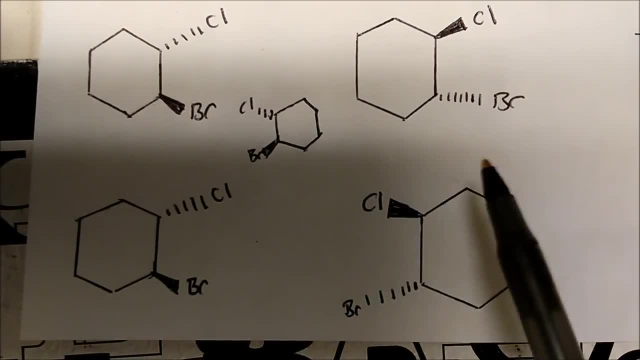 want to get enantiomers, flipping the molecule and changing yourself at your carl centers, that will give you that is basically the same molecule and that is a very important point to illustrate.